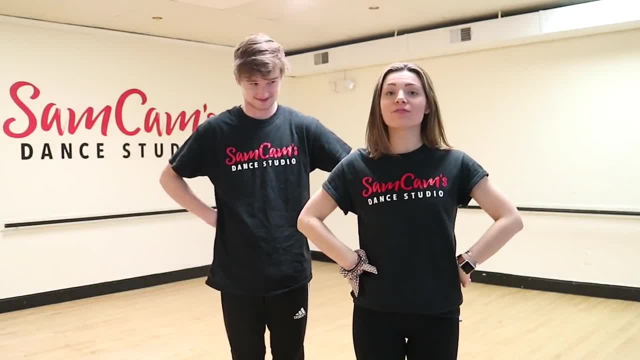 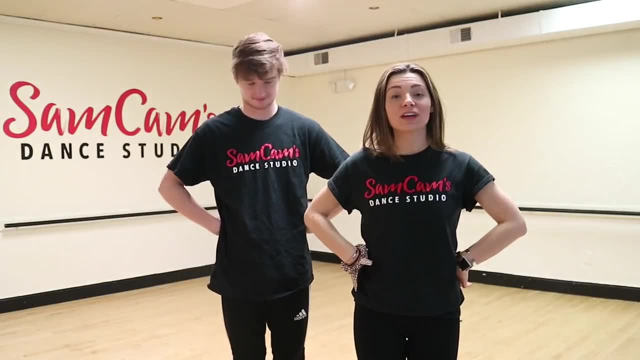 Good job. Rhythm is when we stay with the beat of the music. So what we're going to do is I'm going to make a clapping pattern and Mr Jacob's going to repeat it, And when Mr Jacob repeats it, can you repeat it with him? Alrighty, let's give it a try, Ready? 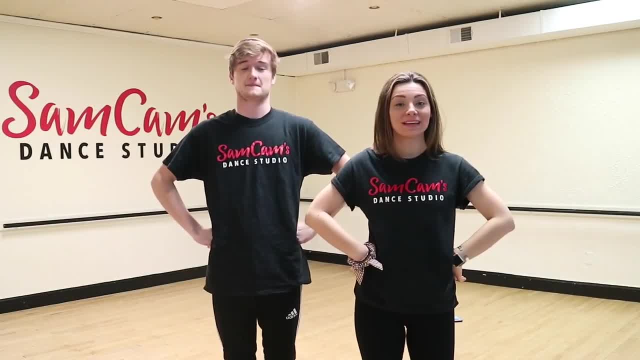 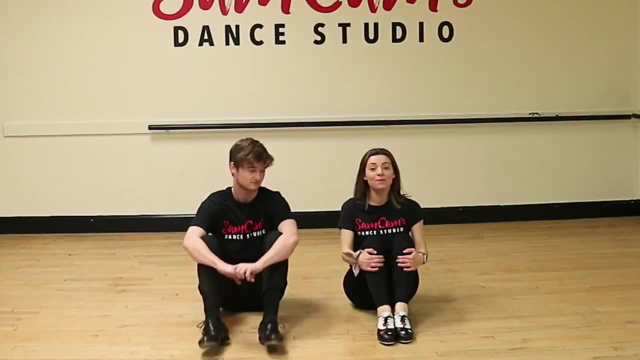 Good job, friends. That was some awesome rhythm and beats. So guess what? I think we're ready to warm on up. Let's get started. Okay, so we're going to start down. We're going to start down on the ground and we're going to give our knees a nice big hug. Good job, Hug those knees, Give them a nice big squeeze. 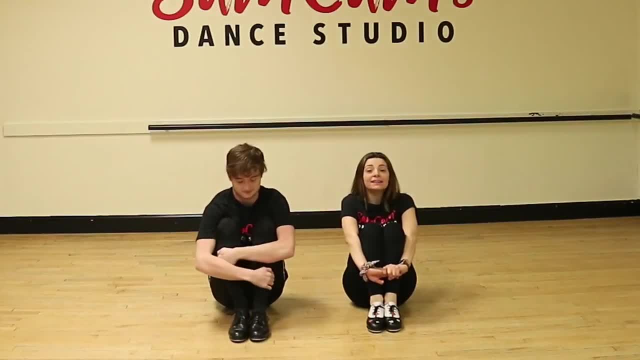 Now ready, We're going to tap our right toe eight times. Can you say right toe, Right toe, Good job. And can you count to eight with me Ready? Here we go: One, two, three, four, five, six, seven, eight, Good job, And give those knees a nice big hug Now. can you say left toe, Left toe, Good job. Here we go, Ready. 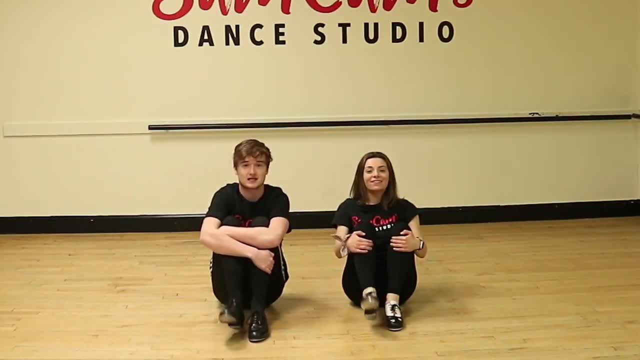 One, two, three, four, five, six, seven, eight, Good job, And give those knees a nice big hug. Now can you say: right heel, Right heel, Good job, Tap that heel. Here we go. One, two, three, four, five, six, seven, eight, And give those knees a nice big hug. Now one more time. Can you say: left heel, Left heel, Good job, Count with me Ready. 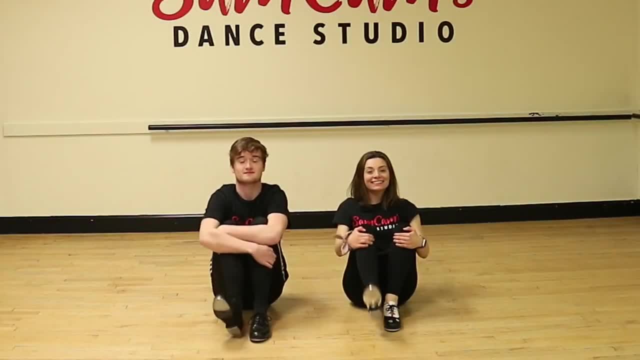 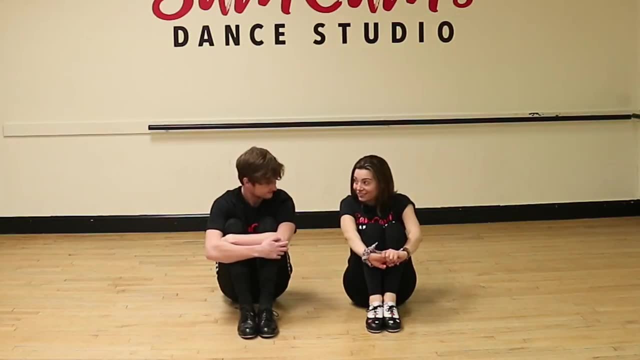 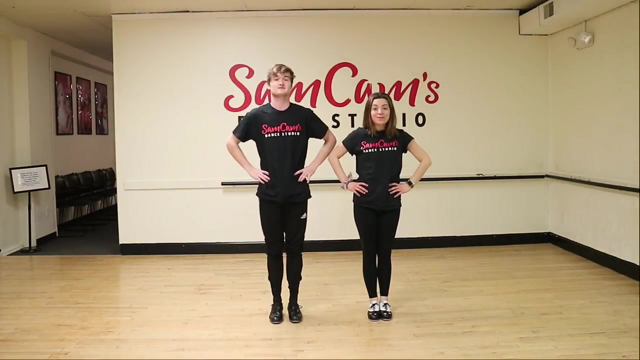 One, two, three, four, five, six, seven, eight And give those knees a nice big hug. Now can we stomp those feet as fast as we can On your marks, get set, go Good job And hug those knees. Very good, We stand on them And now it's time to do our baby shark song. Are you guys excited for our baby shark song? I am, I know I am. 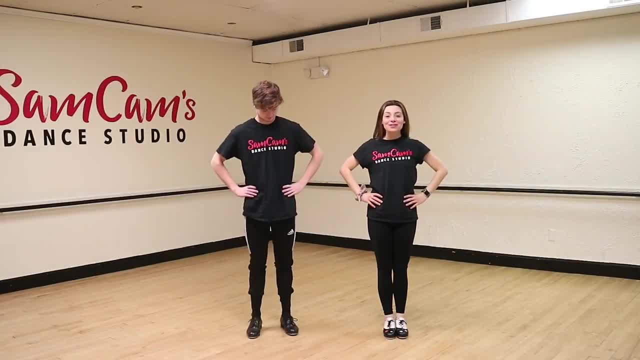 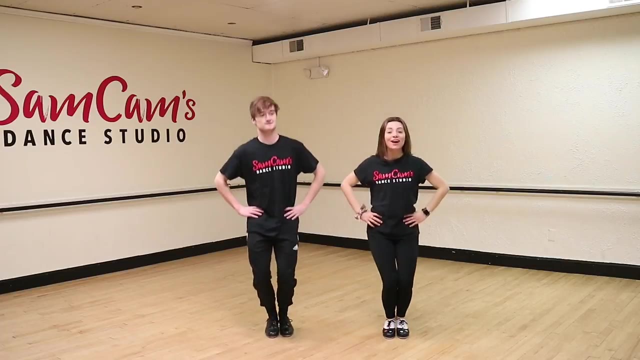 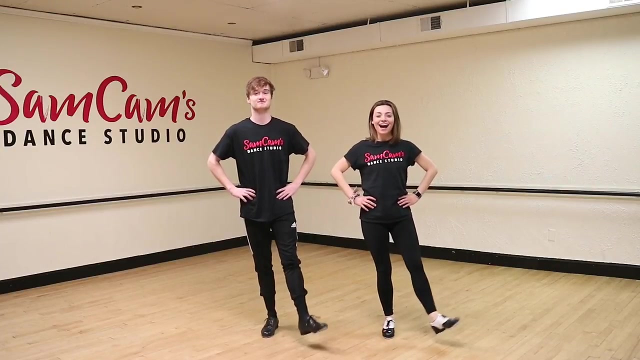 All right, here we go. All right, it's time for our baby shark song. Here we go, Bounce those knees. Good job, All right, we're going to tap our right toe. Here we go. Good job, There is our baby shark. 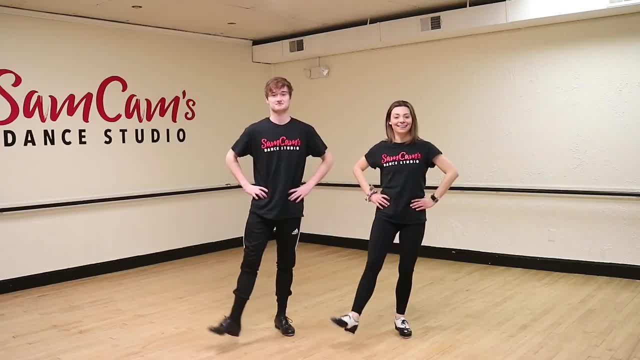 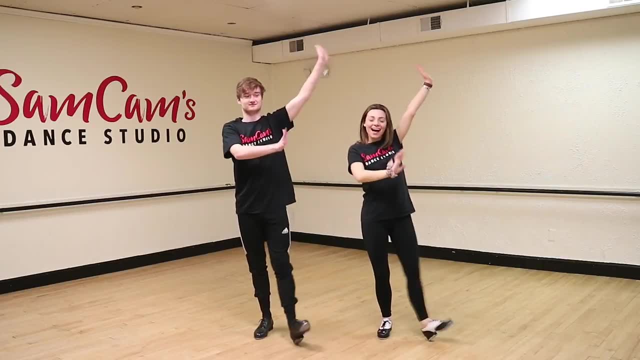 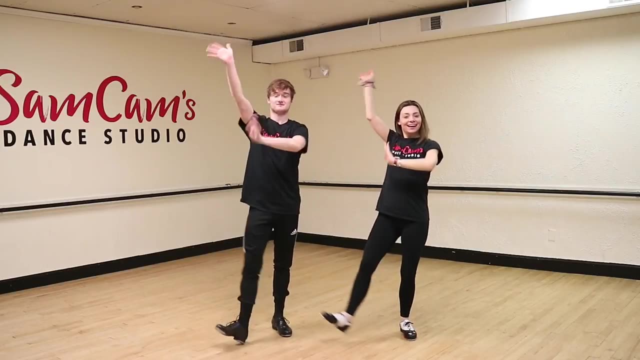 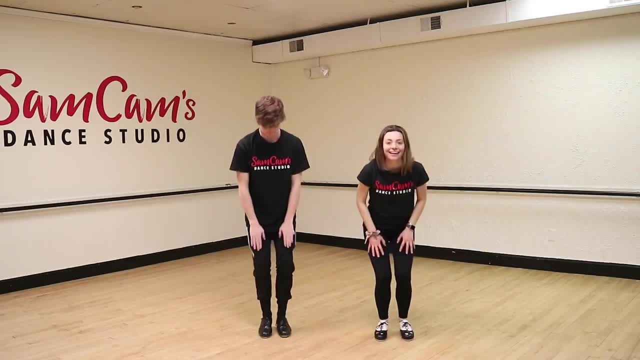 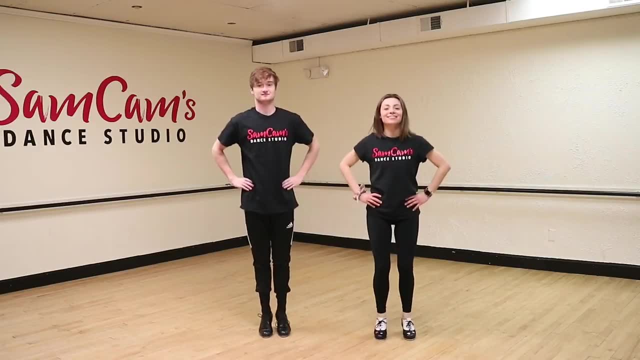 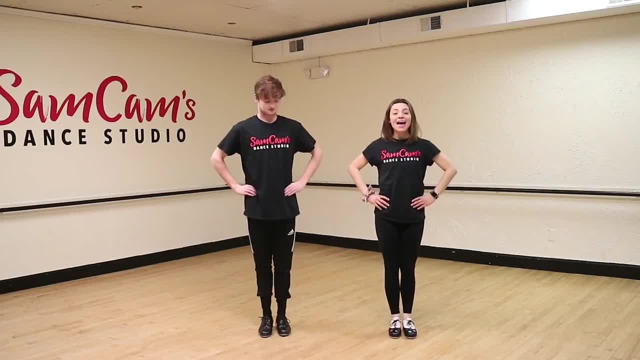 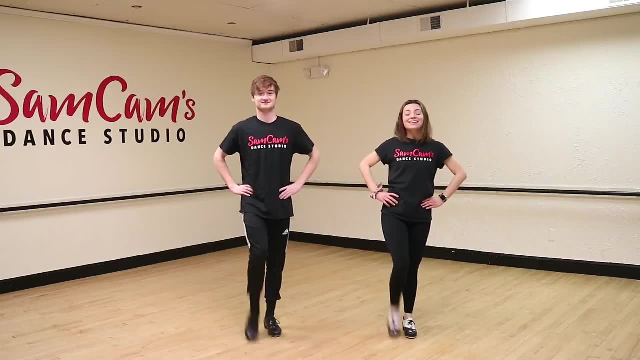 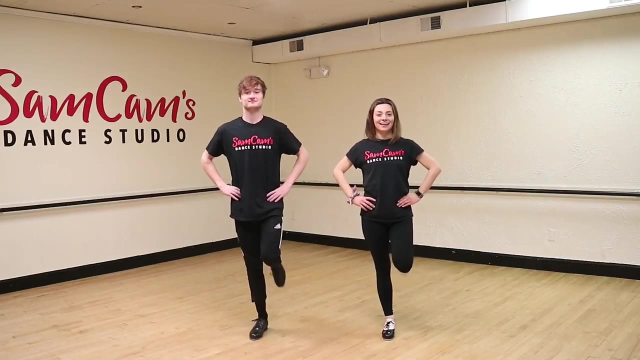 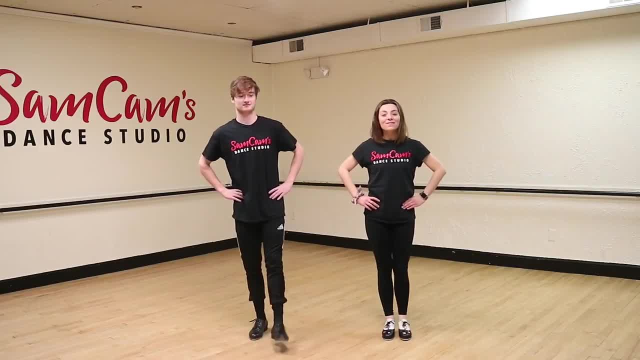 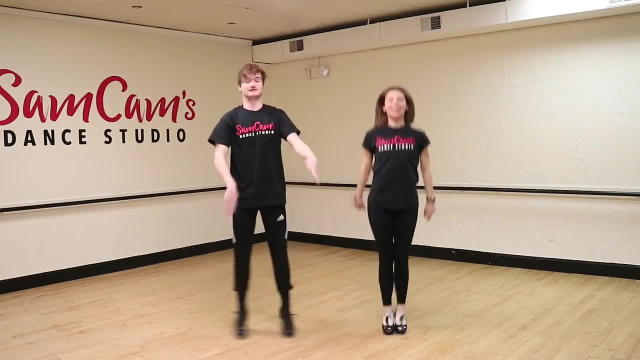 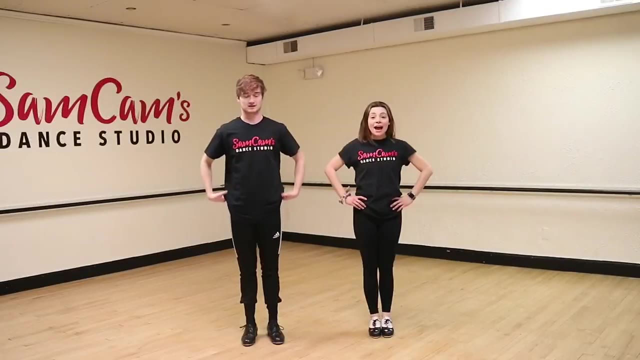 All righty, everybody, we're gonna do balcony And one And one. Oh yeah, you guys are awesome. give yourselves a round of applause. So now it's time to learn the difference between a shuffle and a flap. Can you guys say shuffle, Shuffle? 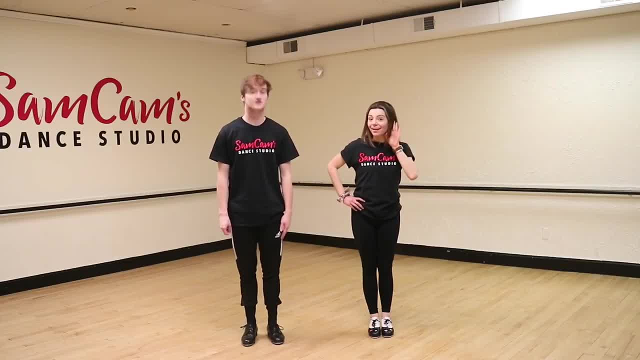 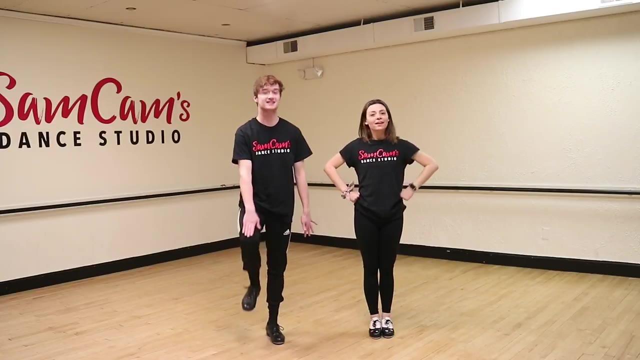 Good job. And can you guys say flap, Flap, Very good. So a shuffle is when we make two sounds and a flap is when we make two sounds. Does anyone know the difference between shuffle and a flap? For a shuffle, you pick up your knee, For a flap, your knee stays down. 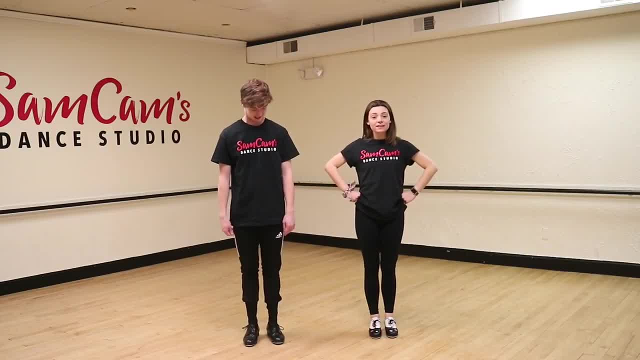 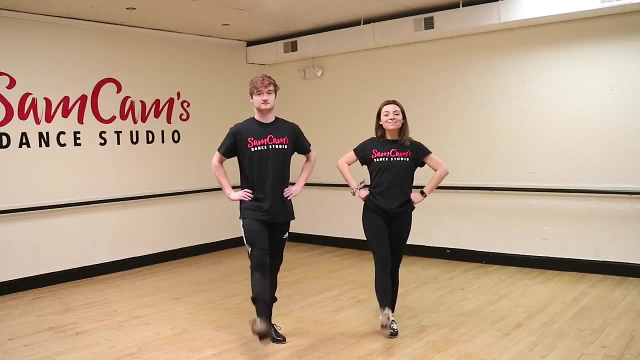 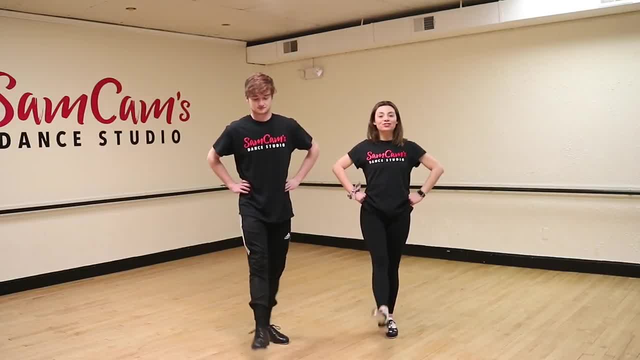 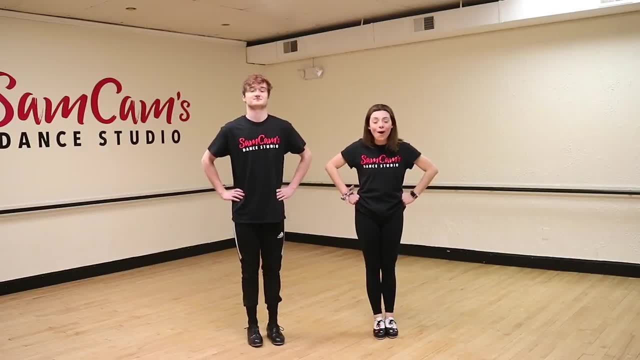 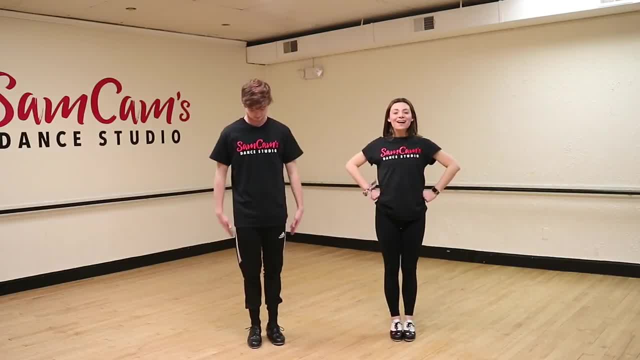 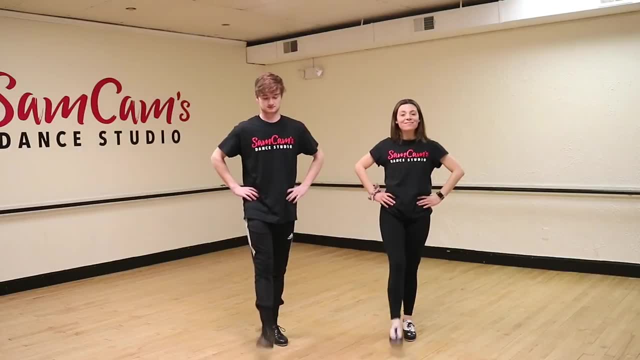 I think so. All right, here we go. Good job, ready, Let's bounce those knees. Good job, let's put those hands right on those hips. Here we go, ready, shuffle And back, back, back, back, back back. 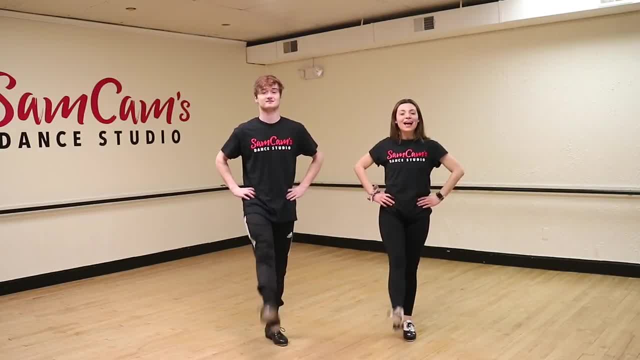 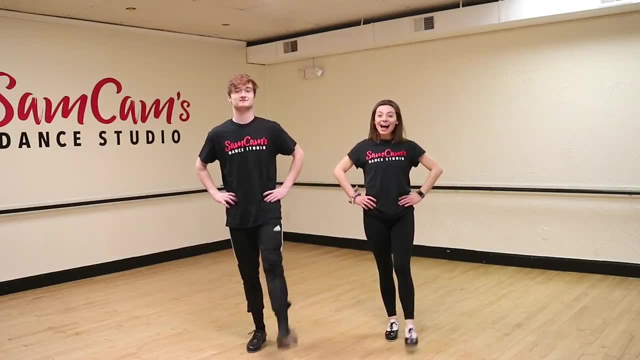 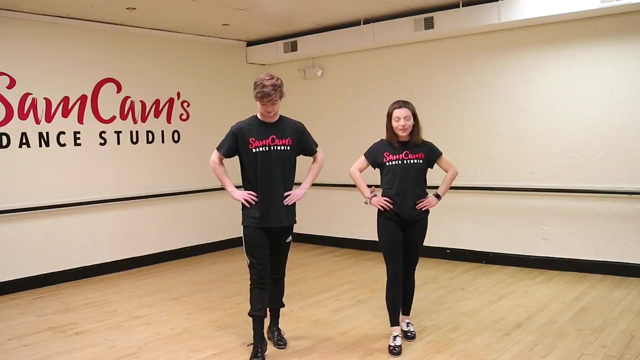 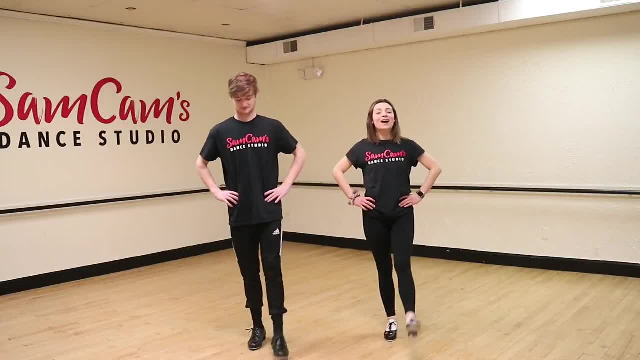 Very good friends And switch. here we go: Front back, back, back, back back, toe, back toe. Good job ready, shuffle, Good job, Very good, and give yourselves a round of applause. 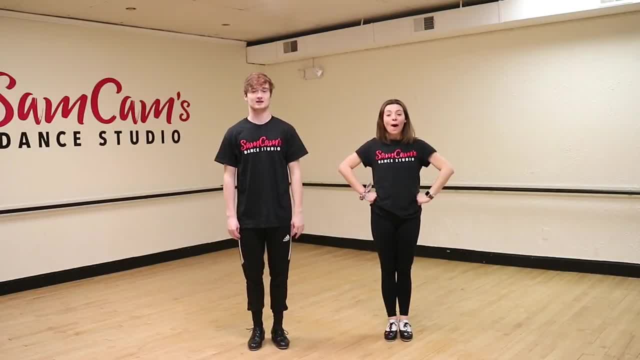 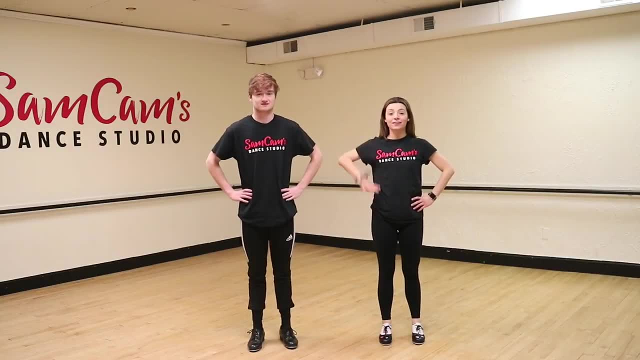 Nice work, friends. that was awesome. All right, so guess what? It's time to learn what a paradiddle is. We're gonna practice a four-count paradiddle today. Can you say paradiddle, Paradiddle. Nice job friends. 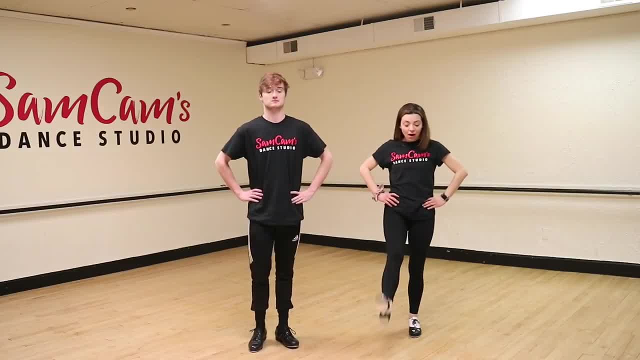 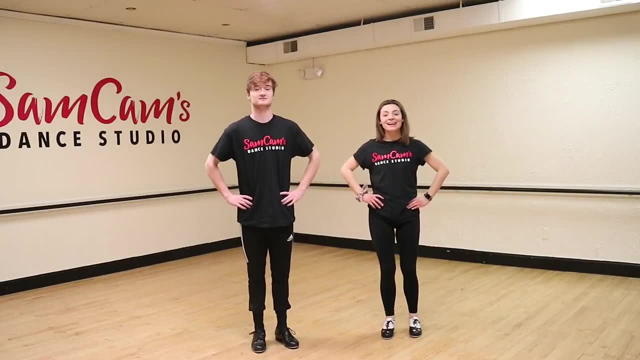 So a four-count paradiddle sounds like this: We're gonna dig our field, We're gonna dig our field, We're gonna pull our foot back and we're gonna tap our toe and then our heel Ready, Heel, pull, toe and heel. 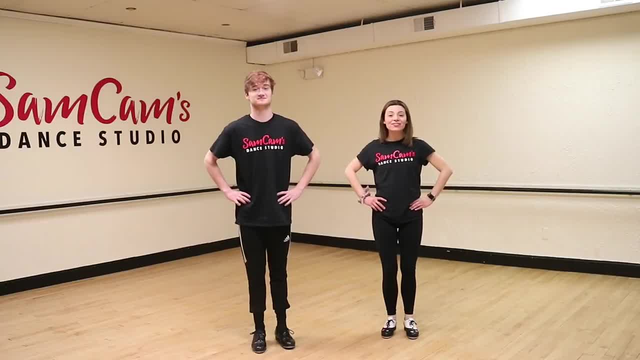 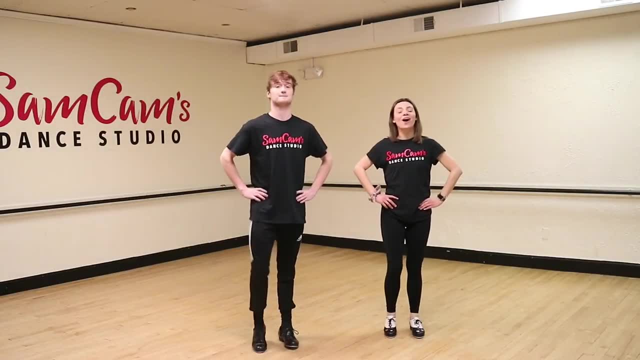 Heel pull toe and heel Say it with me: heel, pull toe and heel. One more: heel pull toe and heel. Nice job, friends. We're gonna follow along with our paradiddle song. 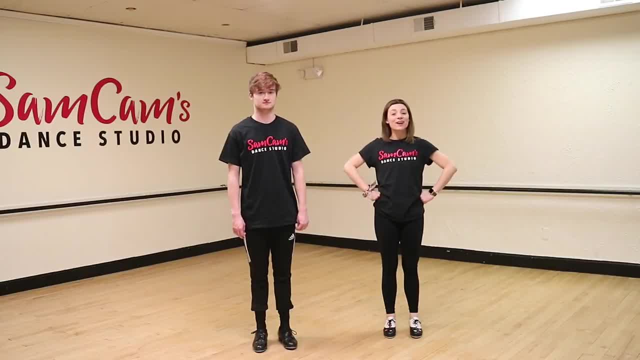 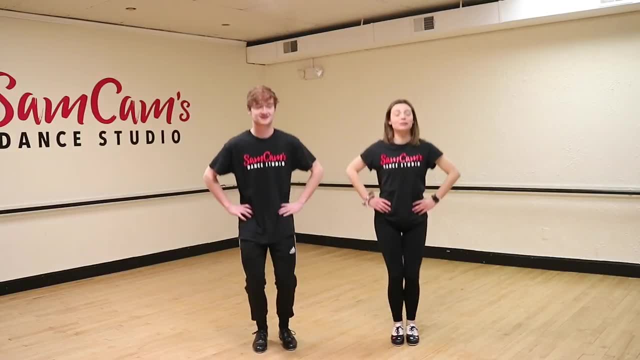 We're gonna go super slow and then we're gonna go super fast. All righty, I think we're ready. Here we go. Good job with those hands right on those hips. That's those knees. Good job, keep those knees super fixed. 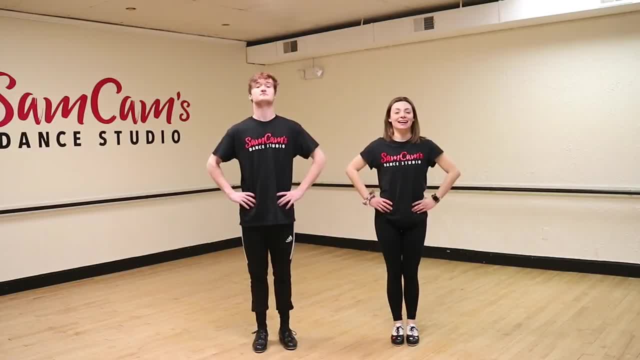 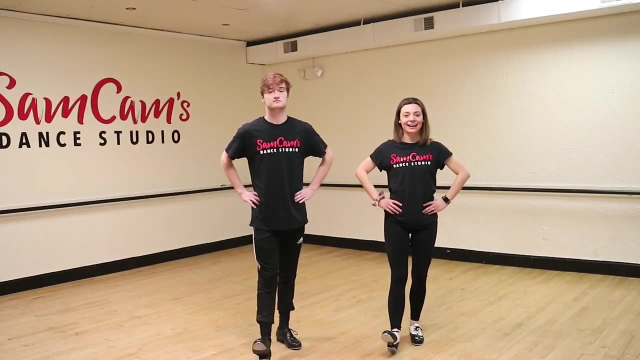 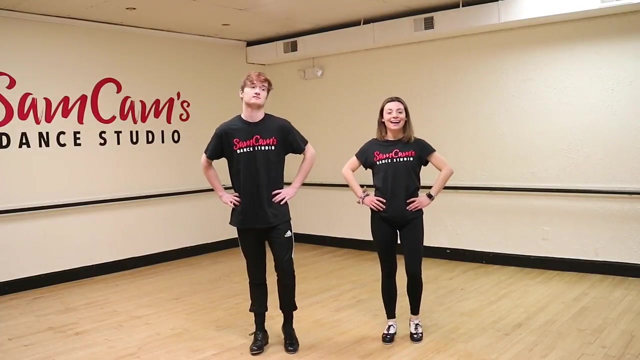 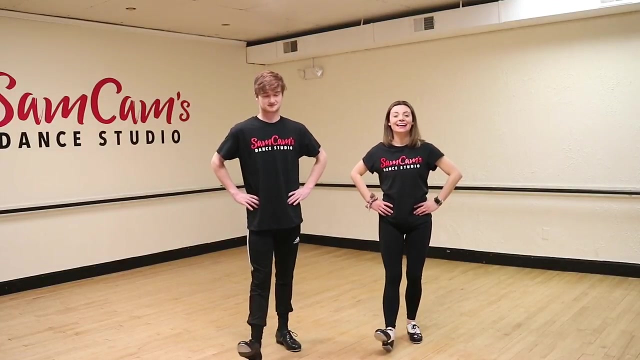 Very good, All righty, here we go Ready. five, six, seven, eight, Heel pull toe heel. Good job, Very good. Good job, Very good. Jump now faster. All right, here we go. 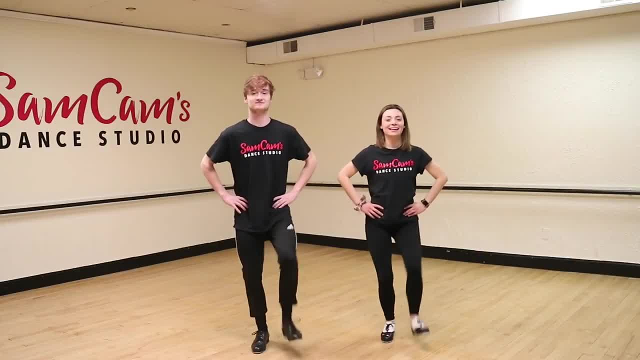 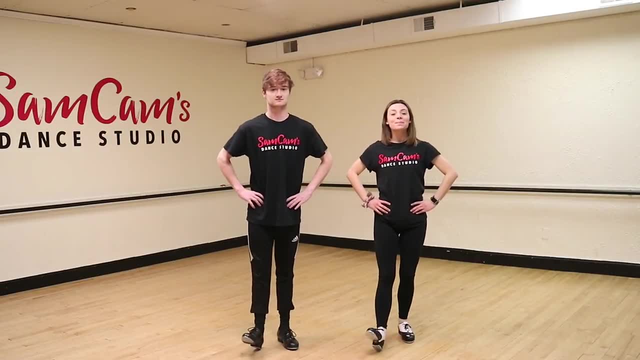 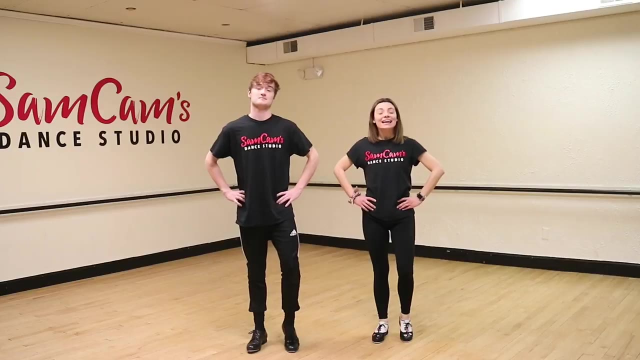 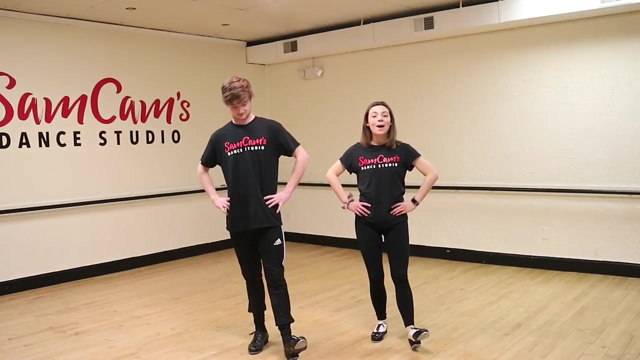 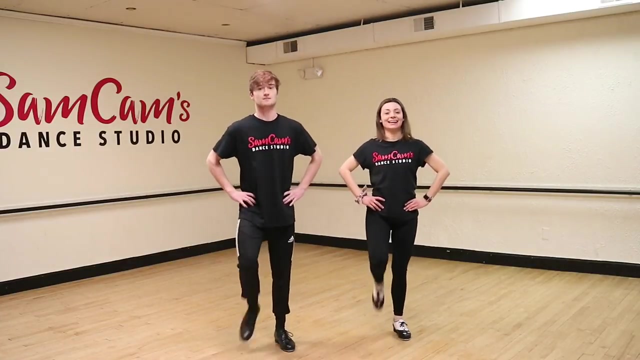 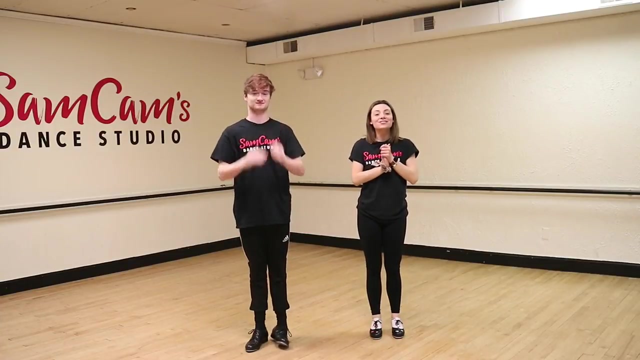 Good job, You can do it, baby. Good job. Good job. Good job, Big push toe, big push, toe, heel, big push. now faster, here we go. good job, now faster, here we go. nice job, friends. give yourselves a round of applause. awesome job, that was some really. 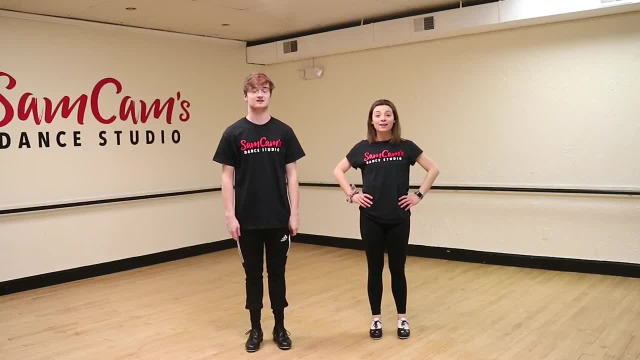 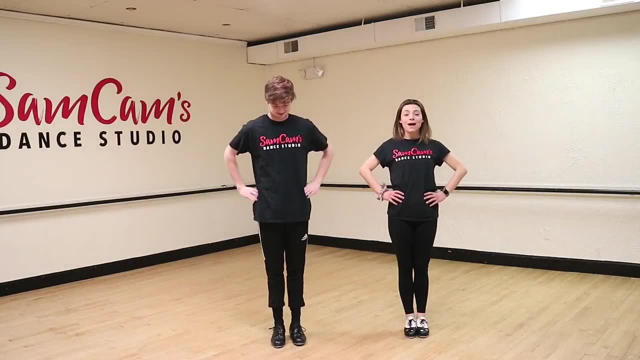 good paradiddles. can you guys say that word one more time? can you say paradiddle, paradiddle. nice job, Mr Jacob. alright, so we're going to start. with those hands on our hips, we're going to do 8 big bounces. can you count with me ready? here we go. 1, 2,, 3, 4,, 5,, 6,, 7,. 8,, 9,, 10,, 11,, 12,, 13,, 14,, 15,, 16,, 17,, 18,, 19,, 20,, 21,, 22,, 23,, 24,, 25,, 26,, 27,, 28,, 29,, 30,. 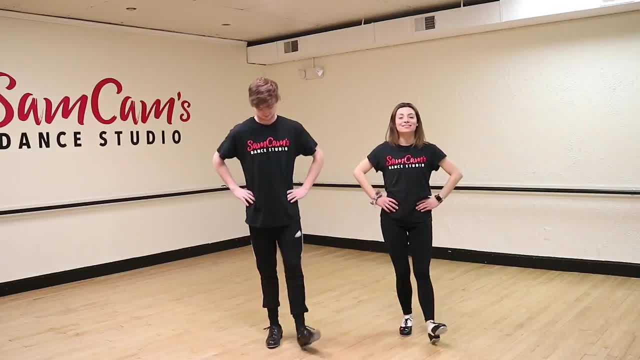 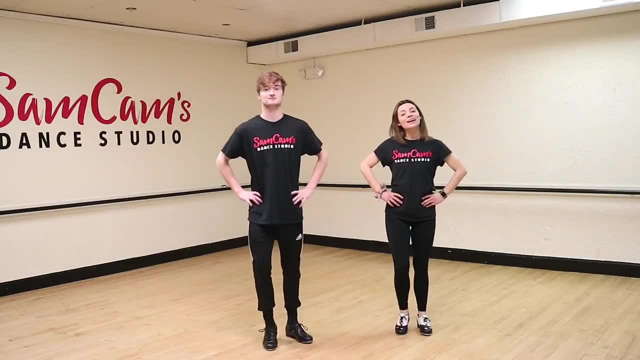 30,. now we're in our paradiddle: 1,, 2,, 4,, 5,, 6,, 7,, 8,, 9, we're going to jump toe, heel, toe, heel, heel. 2, and 3, now we're going to jump in and out. very good, we're going. 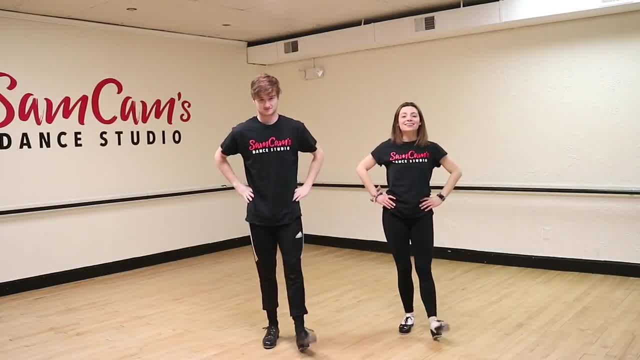 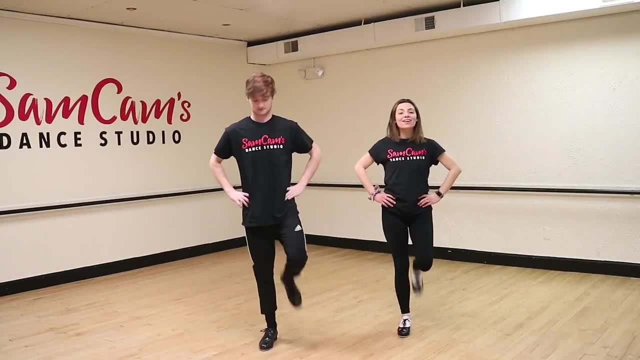 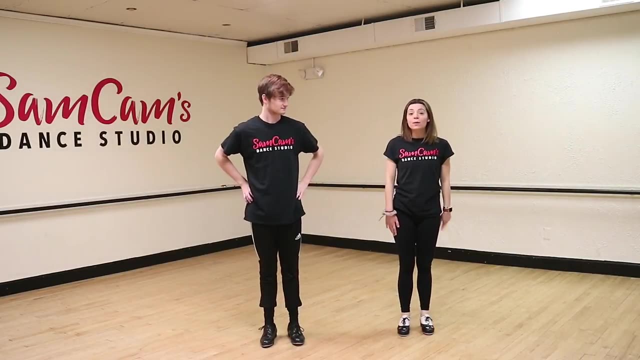 to repeat: ready: heel heel toe heel. good job, very good. now ready our shot toe heel. shot toe heel shot heel. Very good And ready. After our shovel toe kick, we're going to shake one, two, three. 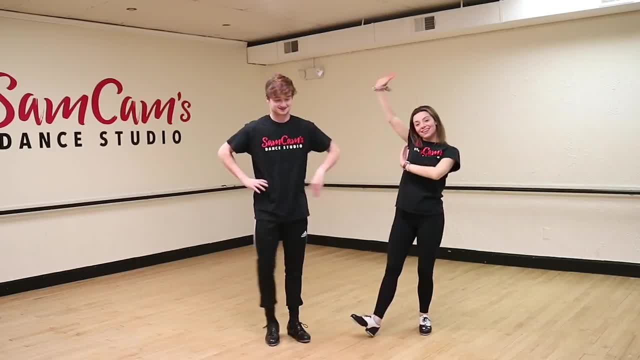 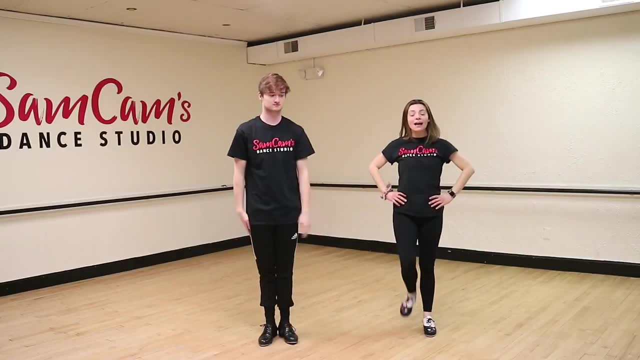 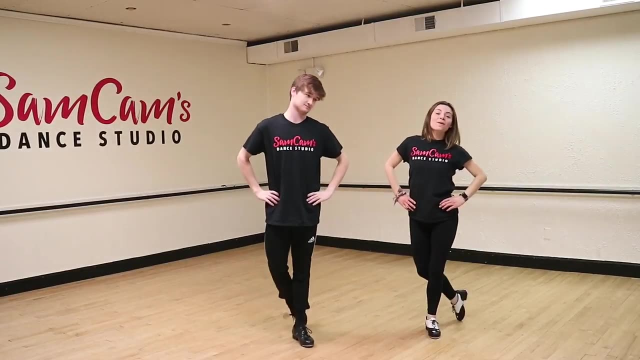 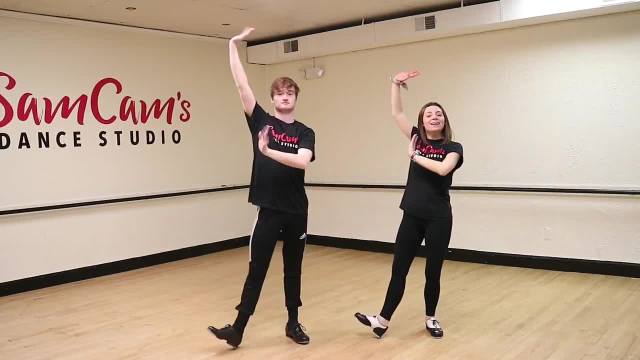 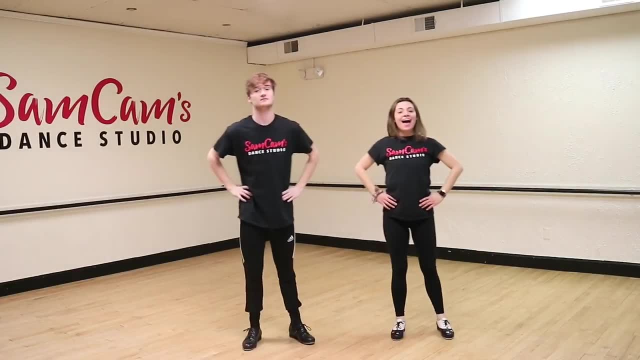 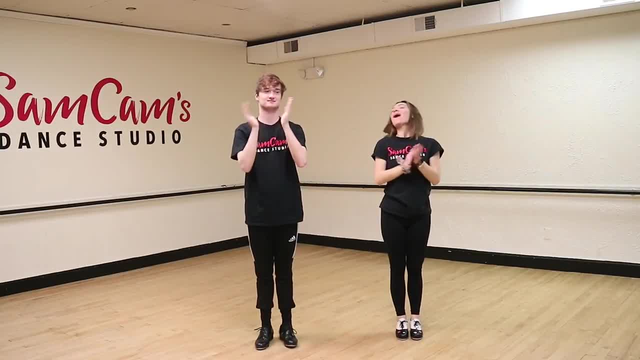 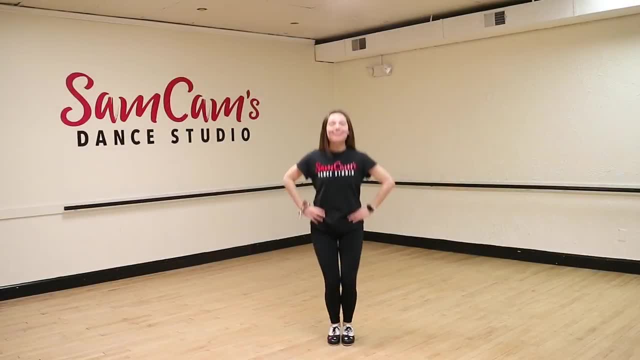 You guys are so cool, Give yourselves a round of applause. All right, Do you guys think that we could try that with the music? I think so. All right, Here we go. Good job, friends, We're going to do a little. 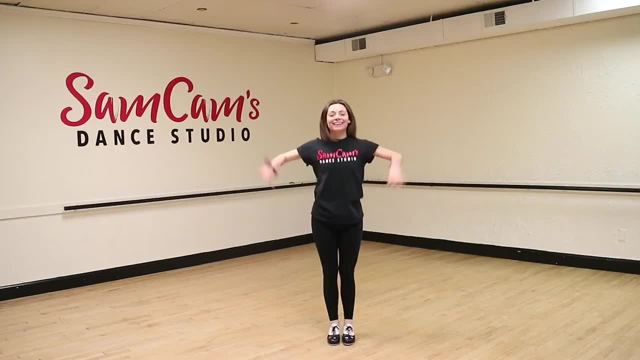 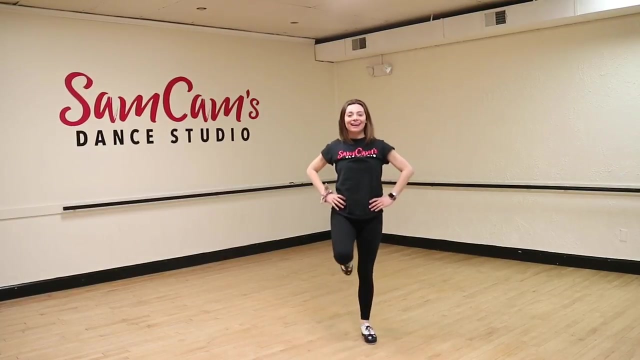 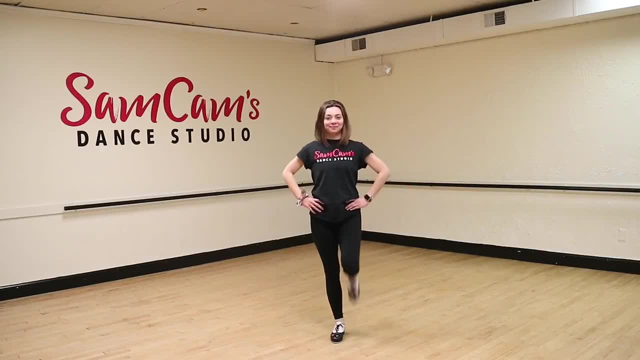 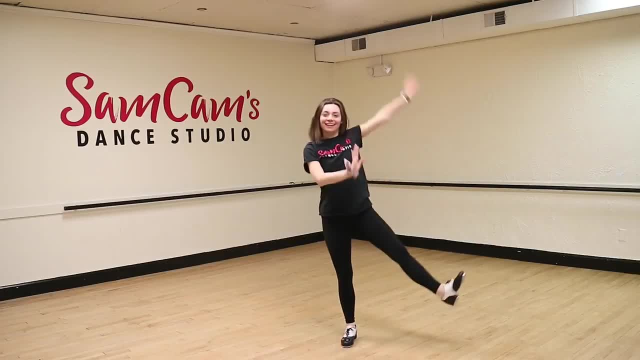 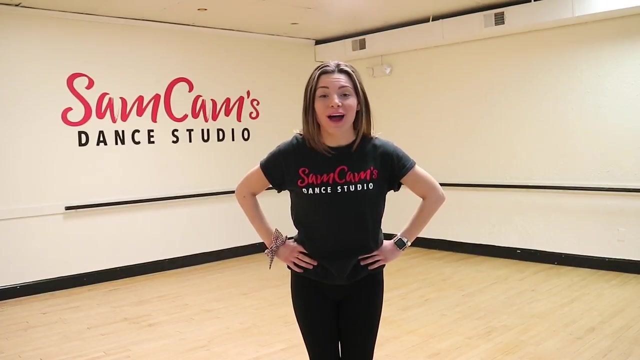 And five: Nice job, everybody. shake those hands all the way back And strike a pose. Nice job, friends. give yourselves a round of applause. Alrighty friends, you guys did an awesome job in tap class today. We are so proud of you. Guess what? Before all dancers leave tap class. 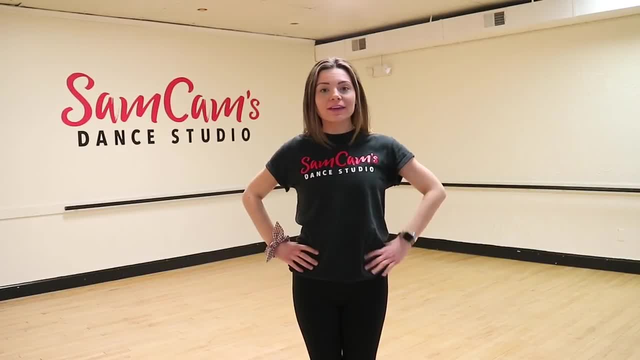 They have to take a really big bow. Can you guys say the word bow? Good job, friends, alrighty. So how many big bows do you guys think we should take today? Did you guys say six big bows? Alrighty, count with me, here we go ready.